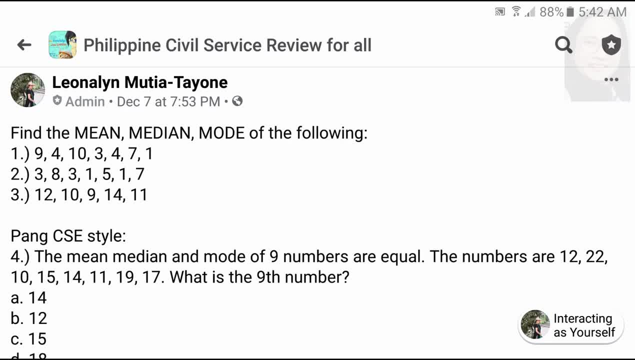 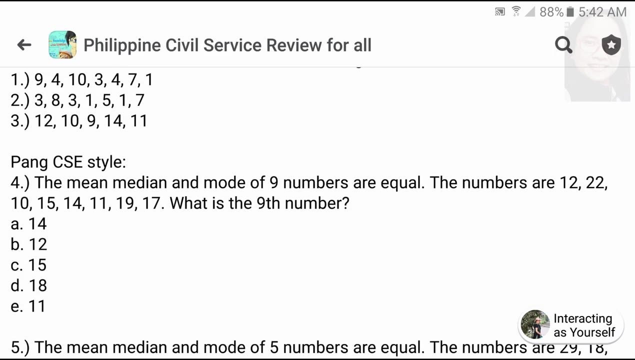 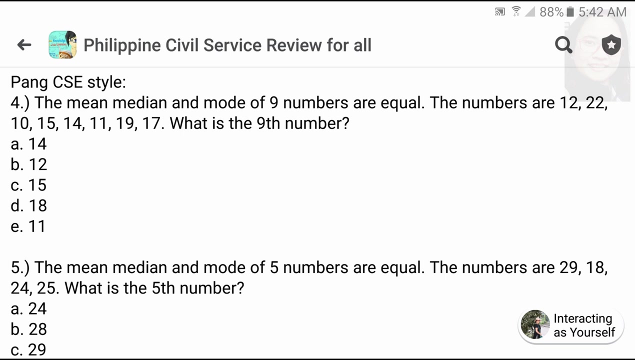 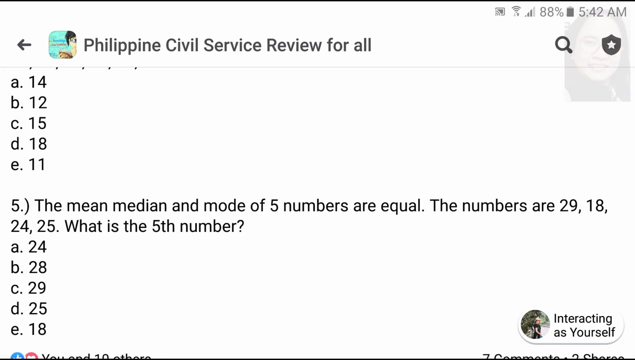 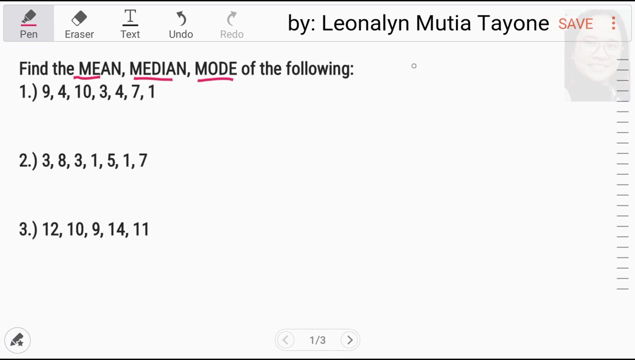 Find the mean-median mode of the following. If you haven't answered them yet, answer them first before you will see our solutions. First, what is mean median and mode? When we say mean, ibig sabihin yan ay average. 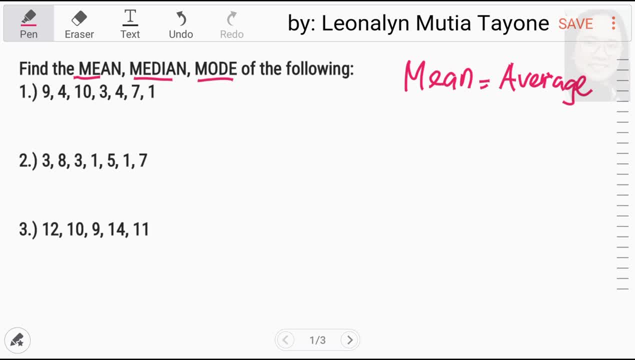 Baka naman hindi namin ibig sabihin yan Kung hindi nyo alam. yung average, that is a number that is calculated by adding quantities together and then dividing the total by the number of quantities. Bali, i-add mo lang lahat, tapos i-divide mo, kung ilan din, yun sila lahat. 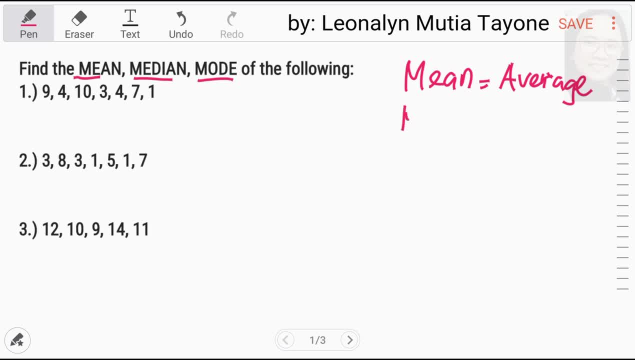 Yan yung average, Next median, When we say median nasa gitna, yan siya Middle, Middle value. Pero dapat i-arrange mo na siya. And then si mode: Yan yung paulit-ulit. 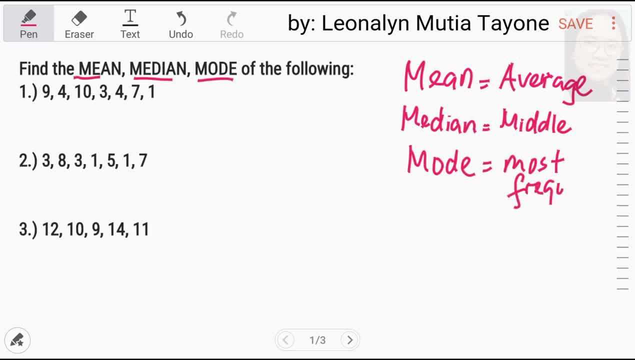 Most frequent Yan si mode. Just in case, hahanapan kayo ng range. Yung range yan yung difference between the lowest and the highest, So highest minus lowest Yan yung range. Question number one: Ang pinakaunang gawin natin ay i-arrange muna natin sila. 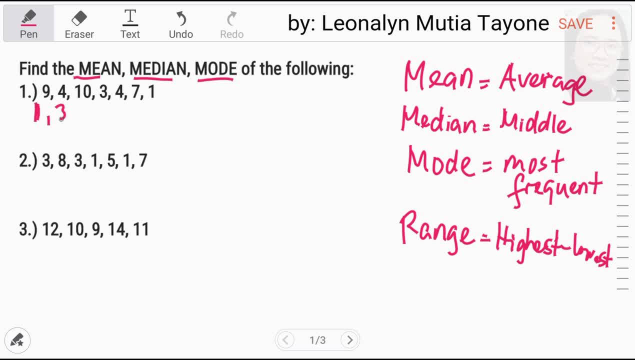 One, One ang una, Next three, Tapos may dalawang, four, seven, nine, ten, I-add muna natin sila lahat. So this is ten, ten, ten, And this one is thirty-eight. 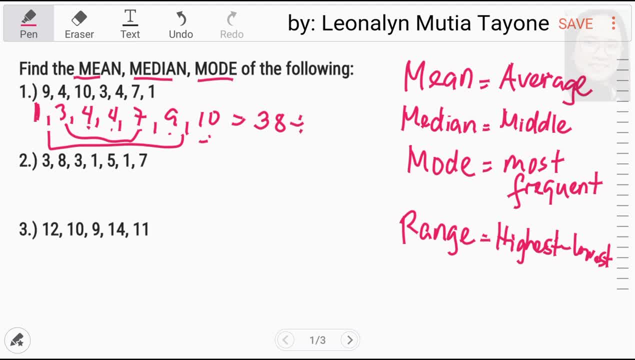 Thirty-eight divided by one, two, three, four, five, six, seven, Seven. So thirty-eight divided by seven, and that is five point four. Kung gusto mong, isa-isahin, isa-isahin natin yan. Thirty-eight divided by seven, 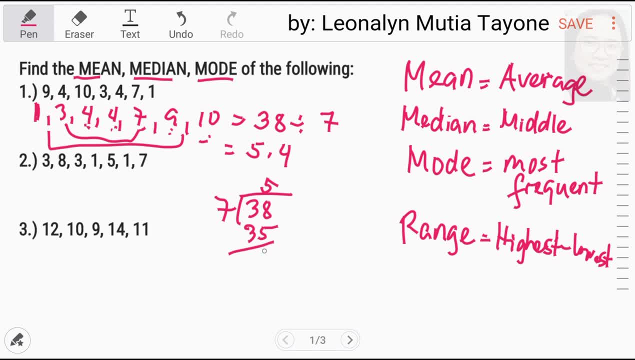 So that is five, Thirty-five. Thirty-eight minus thirty-five, That is three. Tapos maglagay ka ng decimal, kasi magdagdag pa tayo ng isa pang zero. So isa pang zero. Thirty divided by seven, and that is four, twenty-eight. 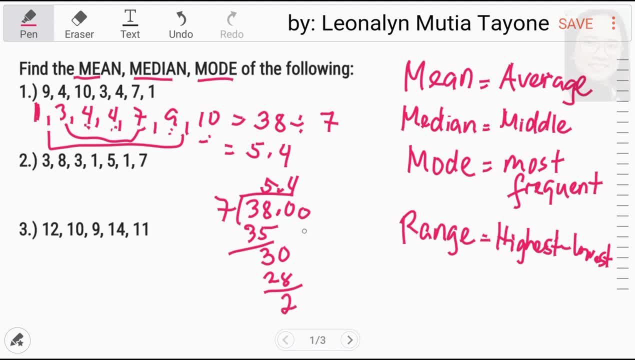 Tapos ito ay two, So magdagdag ka pa ng isang zero. Twenty divided by seven, so two lang yan. Kung sa choices ay five point four, tapos may five point five, dapat mag-solve ka pa until pa mag-add ka pa ng isang zero para makukuha mo yung pangalawa after sa decimal. 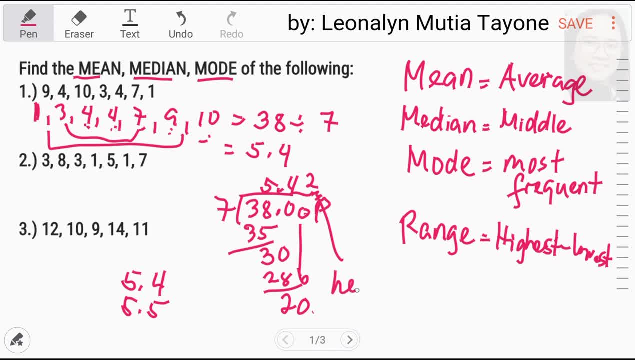 Yung hundreds, hundreds, Hundreds ba ito ba Hundreds yan. So para alam mo kung point five ba or point four, Ngayon, kung sa choices, Kung sa choices ay Merong five point four, two at five point, five at five point. 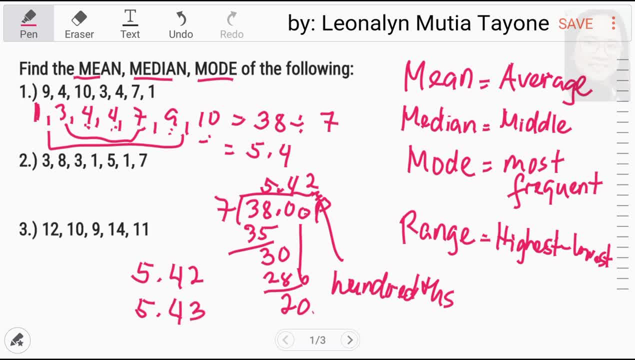 At five, point Ba, 4, 3, kapag ito yung nasa choices, my point 42 at point 43. wag kang mag conclude na ito agad yung sagot, kasi yan yung lumabas dyan. dapat mag add ka pa ng isa pang 0, 20 man yan. oh, so this is 14. 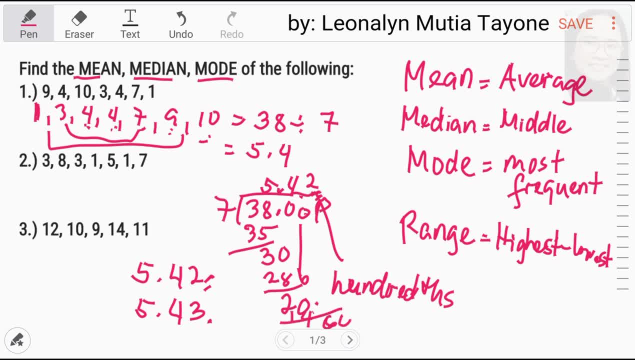 20 minus 14, that is 6. tapos mag add ka pa ng isa pang 0: 60 divided by 7, that is 8. ibig sabihin, kung mag round off ka, magiging 3 na si 2, so ito yung sagot, just in case, kung ang sa choices ay: 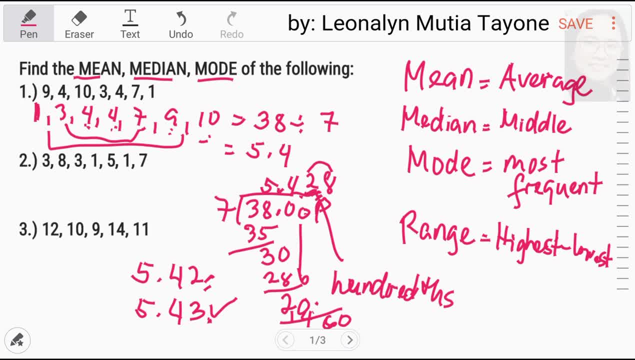 masyadong malapit. point 42 at saka point 43. erase natin yan, kalimutan muna natin yan. dito tayo sa 5.4, so yan na yung average natin. sa number one, ina, add natin lahat ng numbers at dinivide natin. 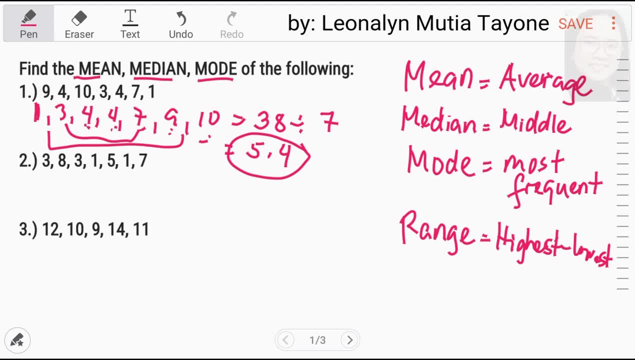 kung ilan sila 5.4. next ay median natin, dito tayo sa gitna, one, two, three, four, five, six, seven, seven sila lahat. so yung yung pang apat, yan yung middle natin. so ito yung middle, yan, yung median natin. next, yung mode, ang pa ulit, ulit most. 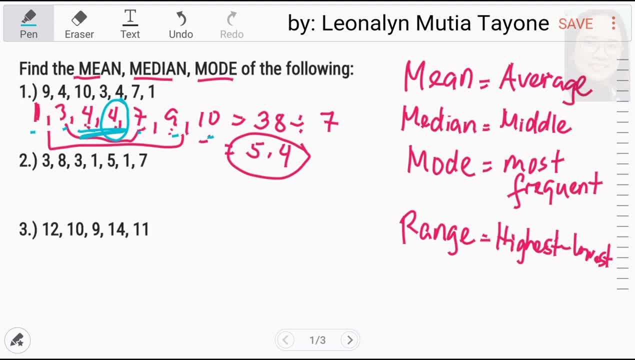 frequent itong si 4. so ang sagot dito sa number one ay 5.4, ang mean natin, tapos ang median ay 4, ang mode ay 5.4. isa pa, kung hahanapan ka ng range, dito tayo sa highest minus lowest, 10 minus 1, and that is 9, yan yung range. 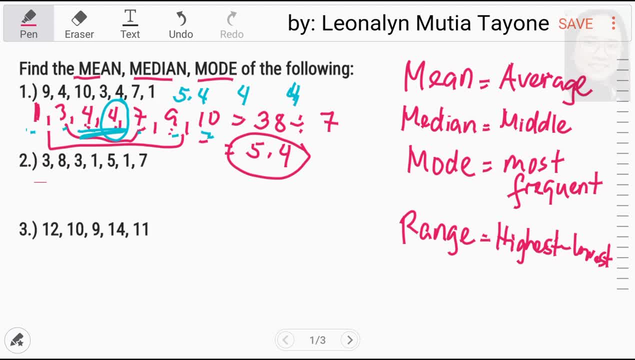 question number two: i-arrange na naman natin ito, so 1, 1, 3, 3, tapos next ay 5, 7, 8 mean. i-add muna natin yung range dito sa highest minus lowest, 10 minus 1, and that is 9, yan yung range. 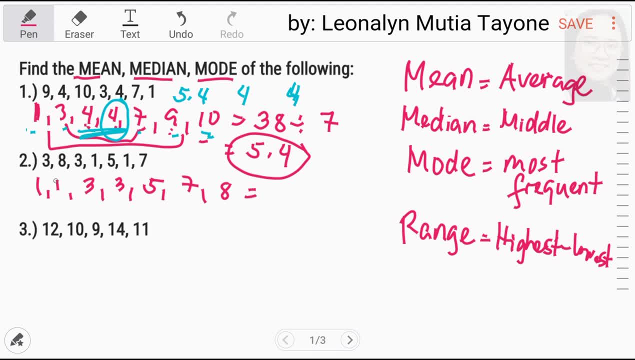 at mornin natin sila lahat at i-divide kung ilan yan ied natin. so this one is one plus one plus three plus three plus five plus seven plus eight plus eight, and this one is ten, tapos 이 kurang is twenty eight divided b'y. kung ilan yan yun is ju pas sa sli po. 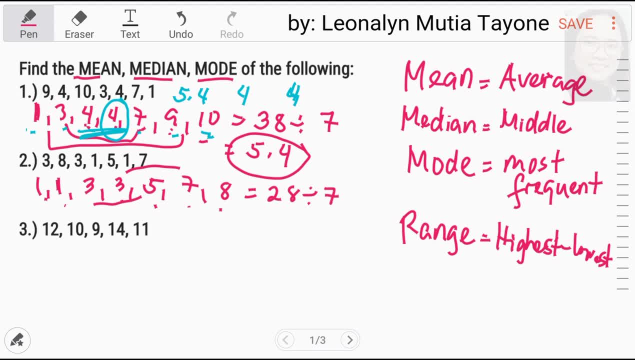 nasa Temperature house perspekt拜 ng Like example: maghanapan mo siya ng partner ba Si 7,. hanapan mo siya ng partner ng 3.. Mayroon man siya Tapos si 5,. hanapan mo siya ng partner ng 5 kung mayroon 5.. 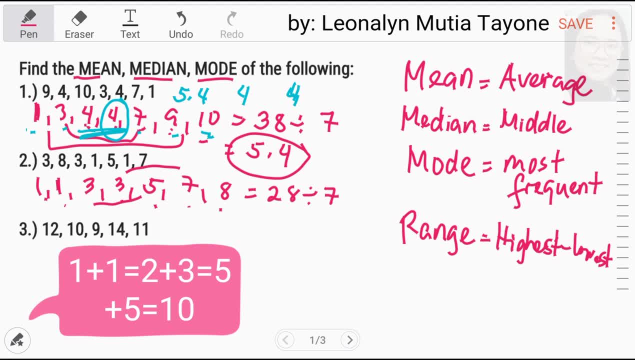 Mayroon man siya 1,, 2, at saka yung 3. 5 man yan siya. So sampu na rin Dalawang, sampu ka na plus 8.. So 28.. Ngayon mean: 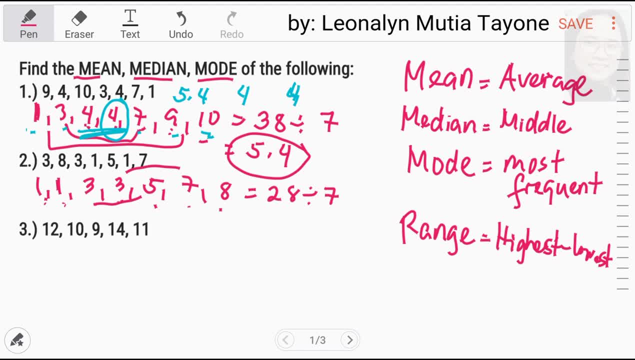 28 divided by 7.. Kasi yan yung 1,, 2,, 3,, 4,, 5,, 6,, 7, sila lahat. So i-divide mo ng 7, yan yung average. 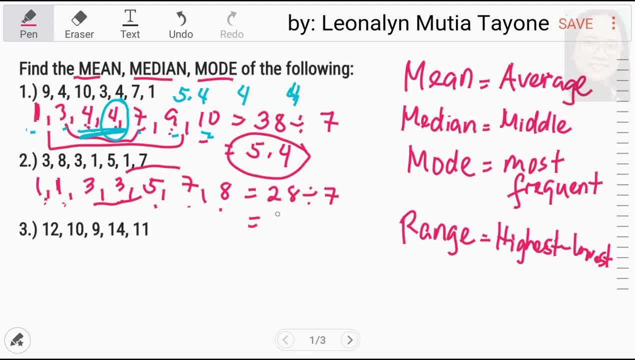 28 divided by 7, and that is 4.. Yan yung mean natin Ang median, yan yung nasa gitna. hanapin natin yung pang-apat 1,, 2,, 3,, 4.. 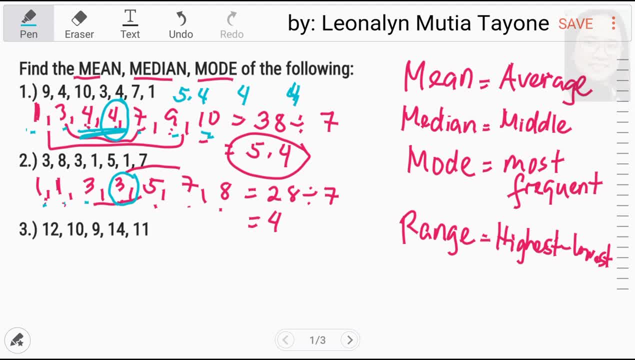 Ito yung median natin Ngayon. dito tayo sa mode Yung most frequent. May dalawa tayong 1. Mayroon din tayong dalawang 3. Alin dyan ang most frequent. 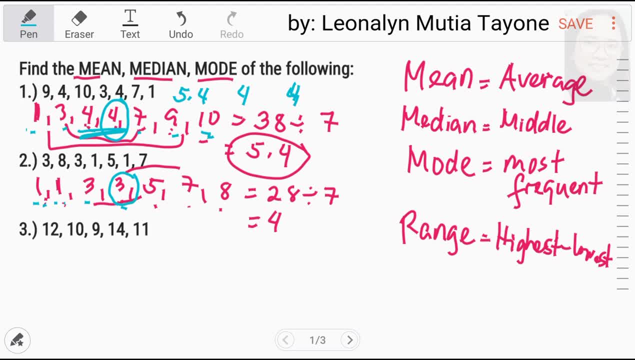 Pareho lang sila. Kaya ang sagot dito sa mode ay 1 and 3.. Next, kung hanapan tayo ng range, Ang range from highest minus lowest, 8 ang highest natin 1 ang lowest. 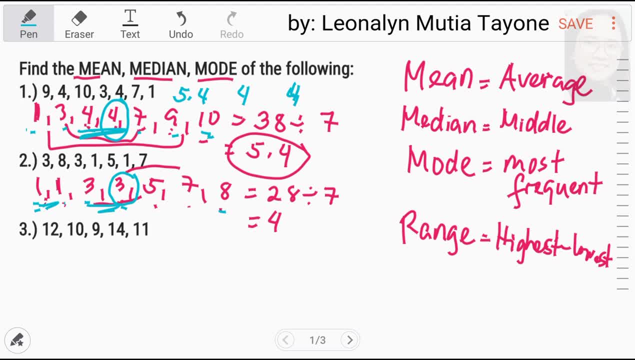 8 minus 1, and that is 7 yan yung range natin. So isa-isahin natin, I-delete muna natin yan. So ang sagot dito ay yung mean natin ay 4.. 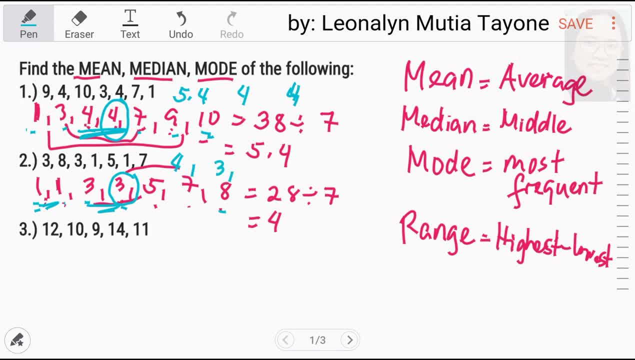 Tapos yung median natin ay 3.. At yung mode naman natin ay 1 and 3.. Mag-recap lang tayo sa 1 and 2.. So ito na yung sagot. I-highlight lang natin. 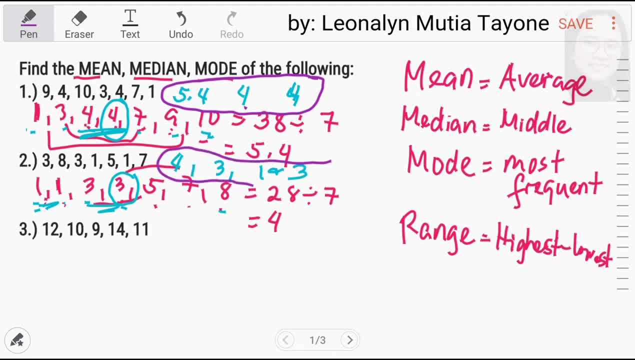 4 ang median, Ang mode naman ay 3.. Dito naman sa isa ay 4 ang mean, 3 ang median, 1 and 3 ang mode Number 3.. I-arrange muna natin ito. 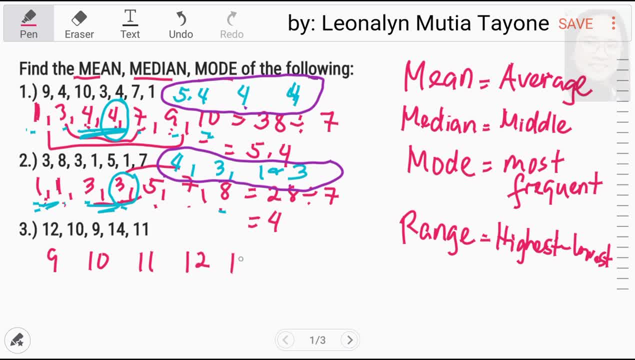 So 9,, 10,, 11,, 12, at saka 14.. Mean I-add muna natin sila lahat at i-divide kung ilan yan lahat. So this is 10,, 20,, 30,, 40,, 56.. 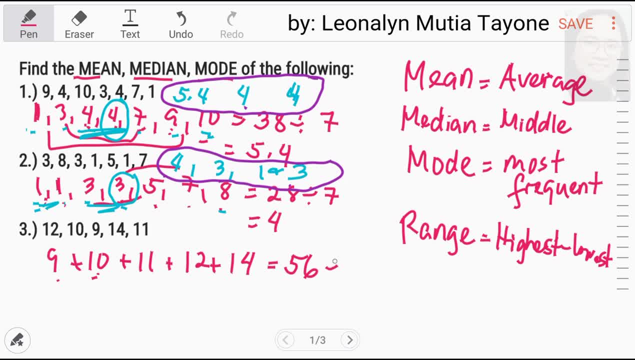 56, divided by 1, 2,, 3,, 4, 5.. Divided by 5, and that is 11.2.. Yan yung mean natin: Median Yung nasa gitna, Ito yung nasa gitna. 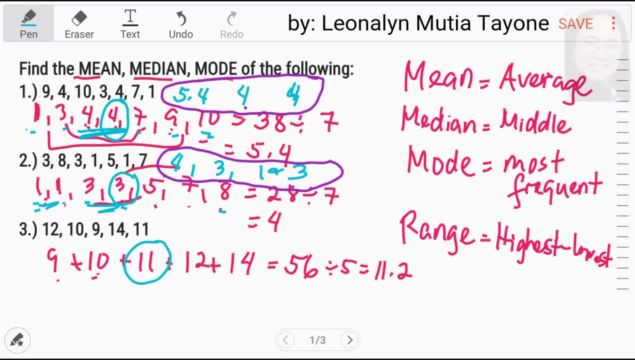 So that's 10.. 11. Mode Pa ulit-ulit or most frequent Sa given May mode ba tayo Wala. So ang sagot dyan ay none, Or kung ano pang synonyms nyo sa wala. basta wala tayong mode sa number 3.. 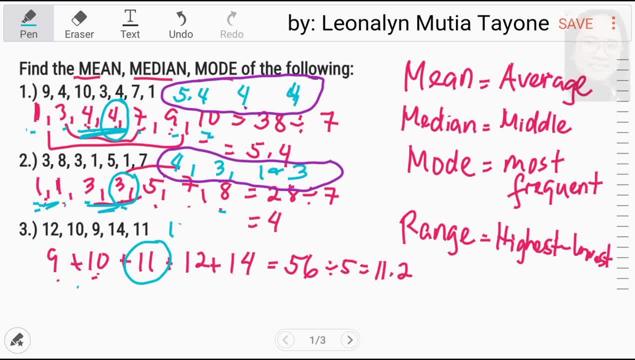 So ang sagot dito sa number 3.. Yung mean natin ay 11.2.. Tapos yung median ay 11.. At yung mode natin ay none. At dagdagan pa natin Yung range. 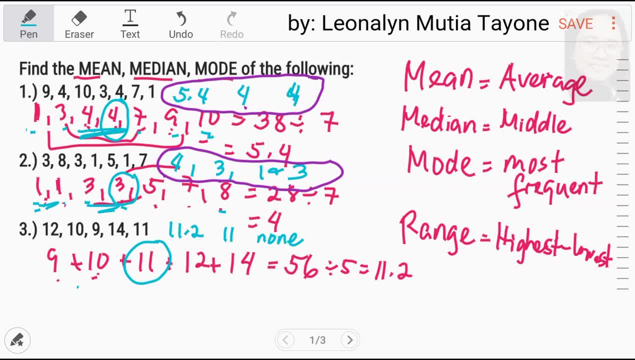 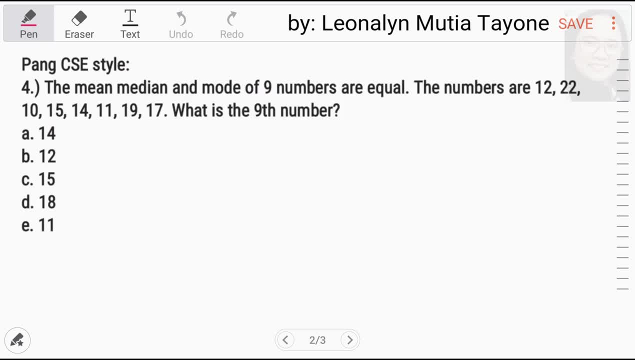 Highest minus lowest. Ang highest natin ay 14 minus 9 equals 5. So yan yung range natin sa number 3.. 5. Number 4. Ito ay pang civil service exam style, At lumabas na ito dati. 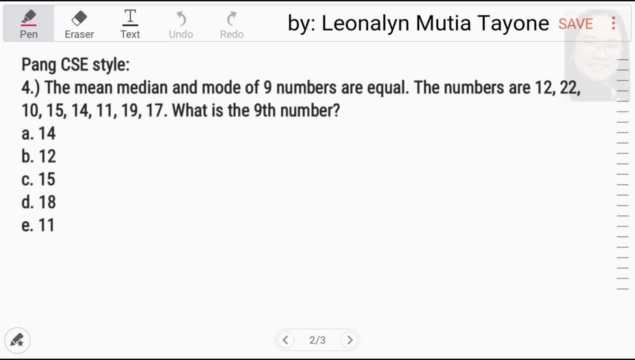 Pero hindi ito yung exact na mga numbers, Pero yung pagkasabi dito yan din yun yung sa previous na civil service na exam. So lumabas din ito Meaning. wag nyong ememorize. 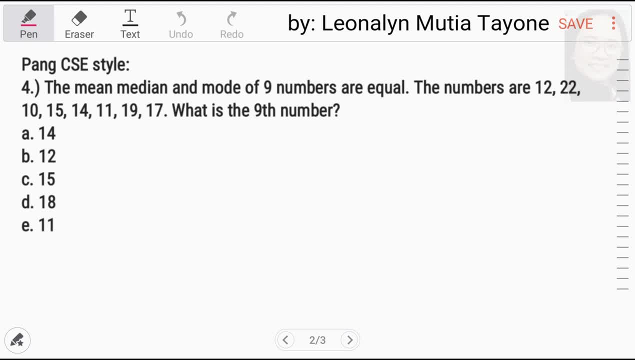 Yung sagot, Kundi yung paraan kung paano ito sagutan ng tama, Para kahit ano pa ang mga numbers ang ipalit nila dito. Kung paano pa man siya ibigay sa inyo yung question? 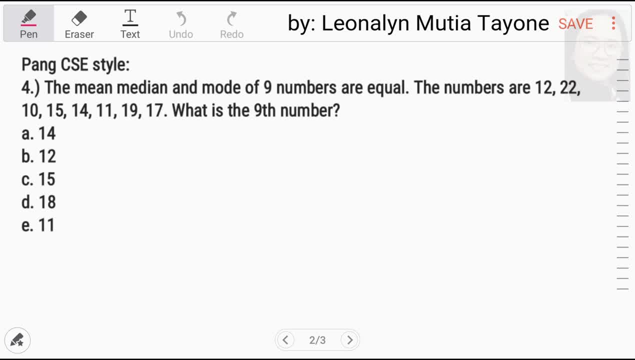 Alam nyo kung paano siya sagutan ng tama, Knowing what is mean median and mode, So dapat mas madali na ito sa inyo. The mean, median and mode of 9 numbers are equal. 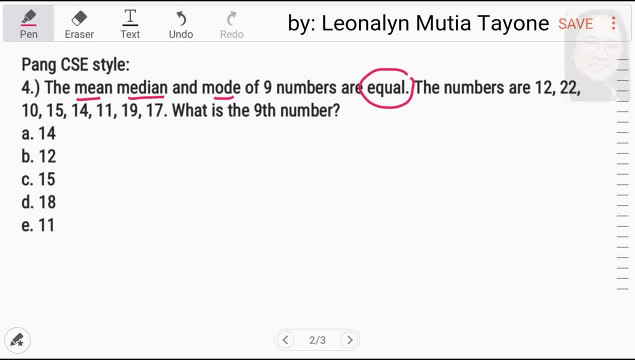 So pariho sila, kung ano man yung mean median and mode Pariho lang. The numbers are 12,, 22,, 10,, 15.. So napansin nyo, kailangan natin i-arrange siya. 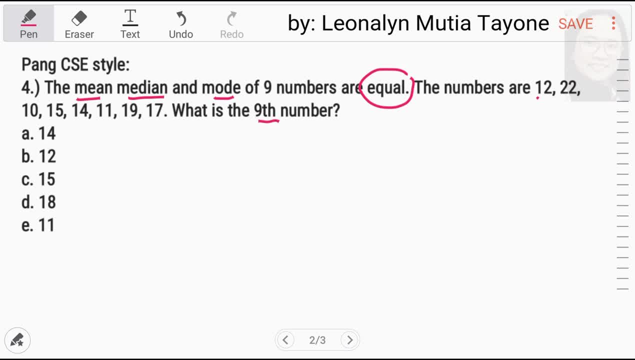 What is the 9th number Sa given? wala pang naulit dyan, Knowing nga ang mode: ayan yung paulit-ulit na number. Kung siya yung paulit-ulit ibig sabihin. 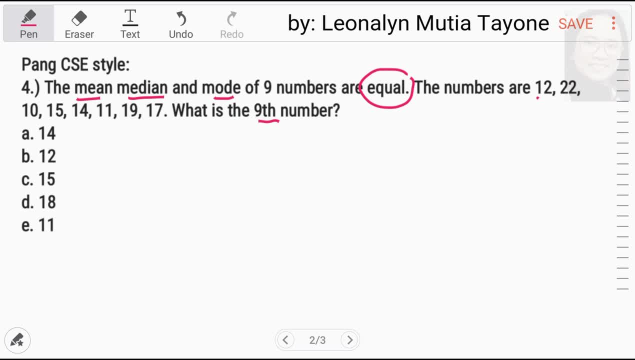 yung 9th number natin ay nandyan lang sa given. Since equal man sila lahat. i-arrange muna natin. Saan ba dito ang pinakamalit: Yung 10,, 11,, 12,, 14,, 15,, 17,, 19,, 22.. 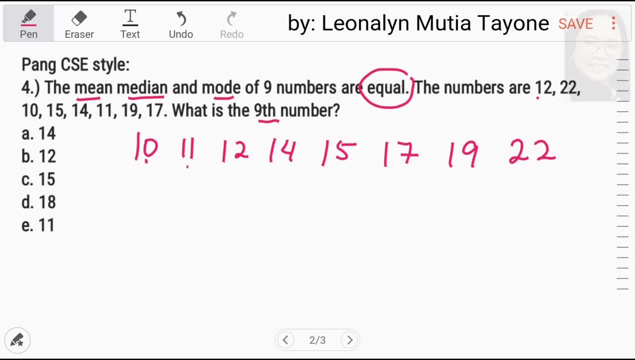 1,, 2,, 3,, 4,, 5,, 6,, 7, 8.. Yung pang 9, yan yung hanapin natin. So kung hanapin natin yung median ngayon, 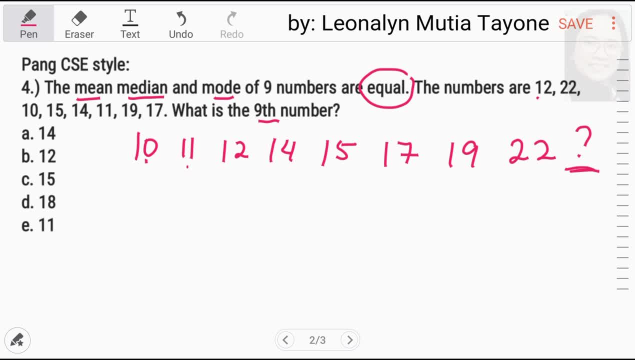 hindi natin alam kung alin dito yung median Ito bang si 15? Asan ang gitna dito: 1, 2, 3, 4, 5.. 1,, 2,, 3,, 4, 5.. 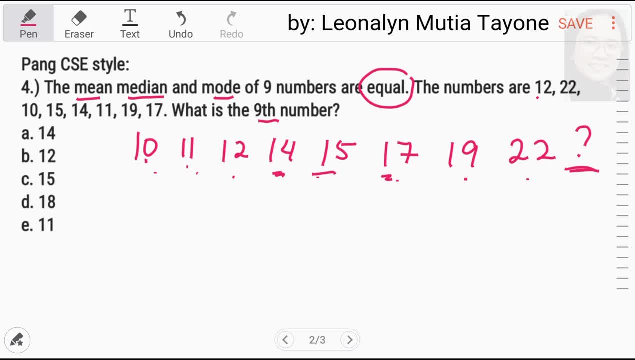 Or pwedeng si 14.. Huwag muna tayong mag-assume na 15 agad yung median natin. Next natin gagawin ay: i-add muna natin sila lahat at i-divide ng 8.. 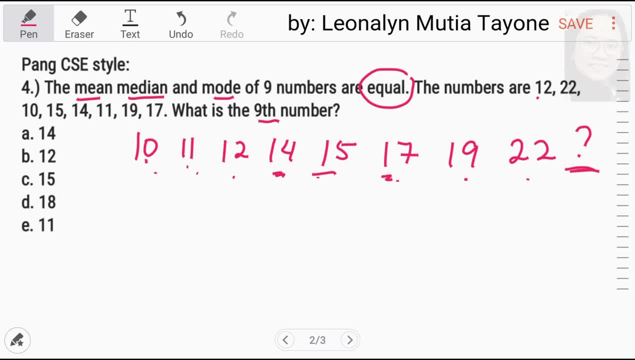 Kasi 8 lang sila Lahat, So mag-average tayo sa 8.. Total ang pang 9th number naman natin yung average sa 8, bali yung pang 9, natin yan din yung number na yun. 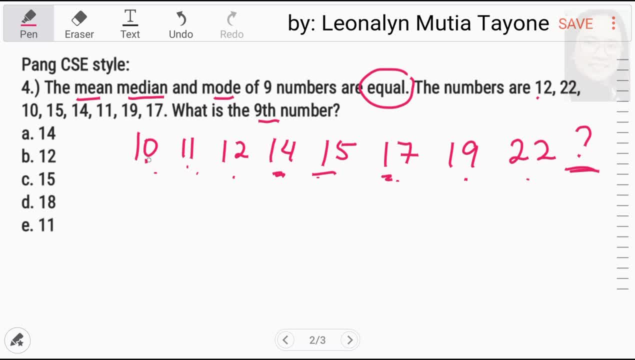 So i-add muna natin So ilang 10 ba to 1,, 2,, 3,, 4,, 5, 6,, 7,, 8, 9.. Mayroon na tayong 90 dyan. 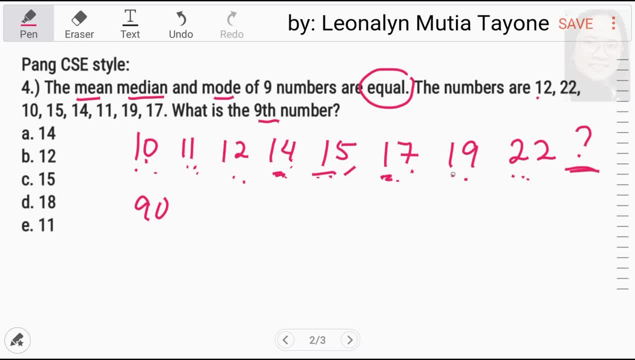 So this one is 3,, 7,, 2,, 9,, 8,, 10.. So 1,, 2,, 3. Equals 120 sila lahat. So 120 divided by 1,, 2,, 3,, 4,, 5,, 6,, 7,, 8.. 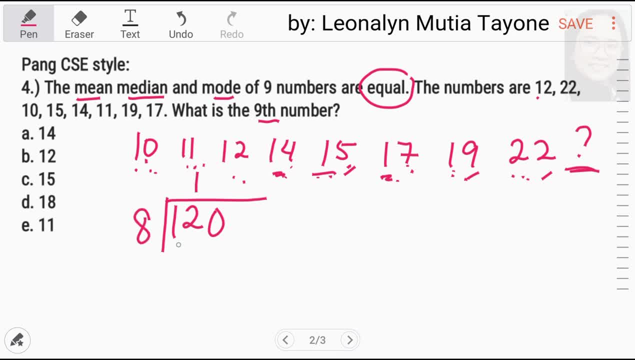 So divided by 8.. So ito ay 1,, 8,, 40,, 5.. 5 yan 40 divided by 8 equals 5.. So ang average natin dito ay 15.. So kung 15 ang average dyan. 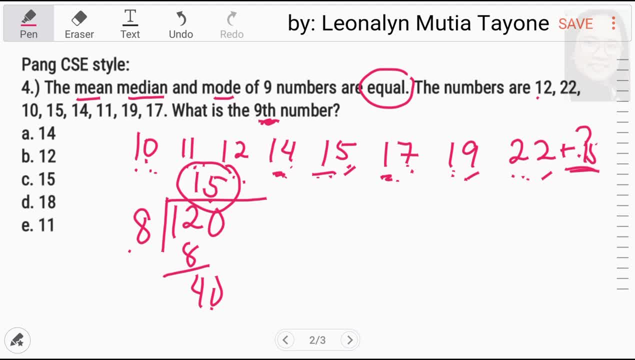 ang pang 9th na number. ang i-add mo pa ay 15.. Tutal, kung i-add mo siya, divide mo ng 9, 15 ang average. Ibig sabihin pwede mo siyang i-15, 15 lahat ba. 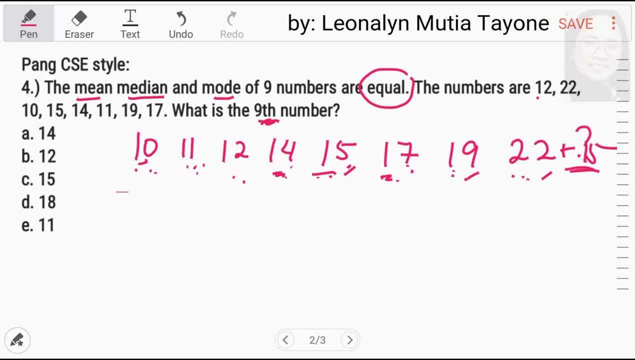 So i-dagdag muna natin yung 15. para klaro sa lahat, This will be 10,, 11,, 12,, 14,, 15, tapos isa pang 15,, 17,, 19,. 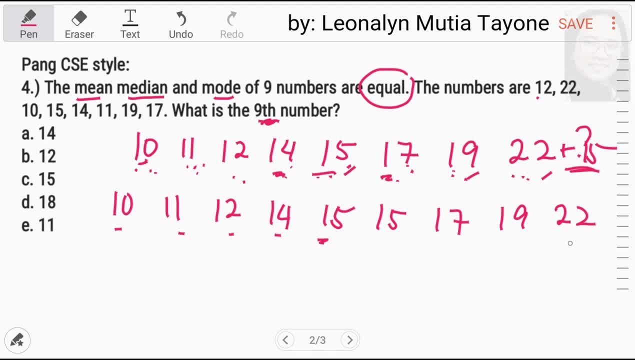 at saka 22.. 1,, 2,, 3,, 4, 5.. So ito na yung nasa gitna Yan, yung media natin, Ang mode natin 15.. Media natin ay 15.. 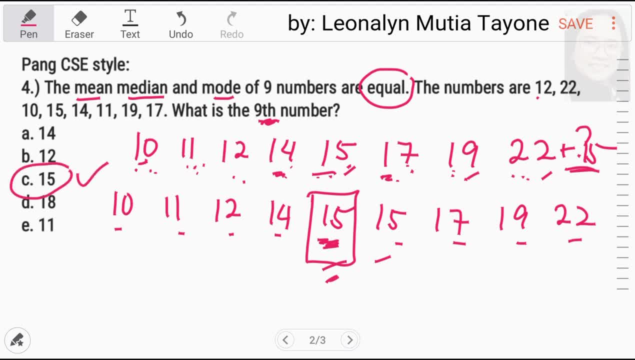 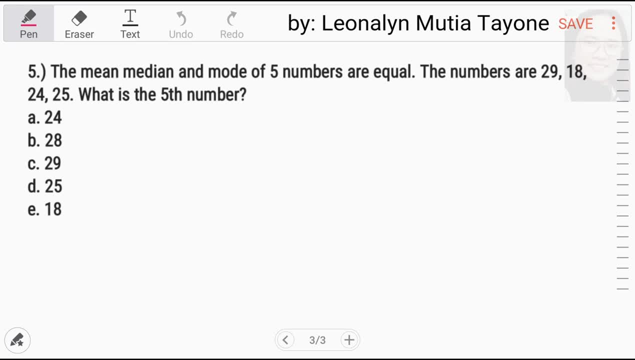 Average niya ay 15.. So ang sagot dito ay letter C. Para mas lalong maintindihan, dito tayo sa question number 5.. The mean, median and mode of 5 numbers are equal. The numbers are 29,, 18,, 24,, 25.. 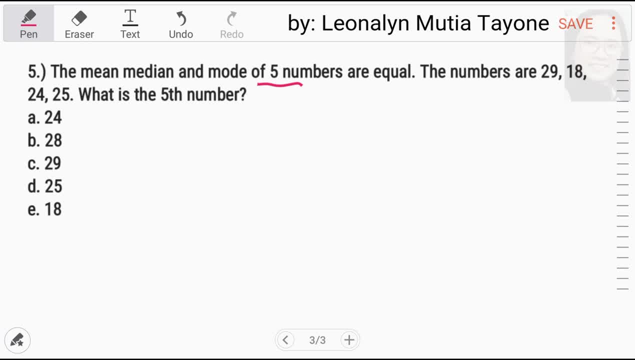 What is the 5th number? I-arrange na naman natin ulit 18,, 24,, 25,, 29.. At hanapin natin kung ano kaya yung panglima Ngayon. huwag tayong mag-assume na 25 siya. 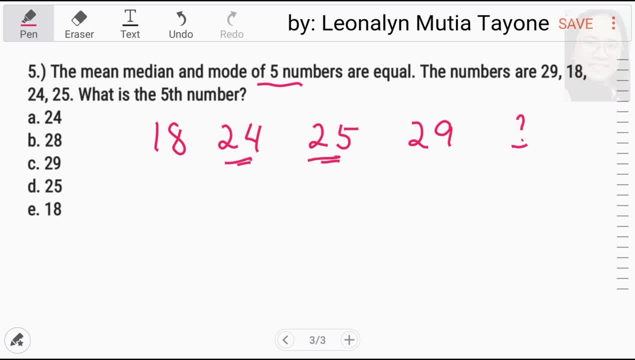 or 24, yung median natin Mas safe kung i-add muna natin yan at i-divide ng 4.. So we have 50,, 70.. 8 plus 4, 2.. 7, 6, 26.. 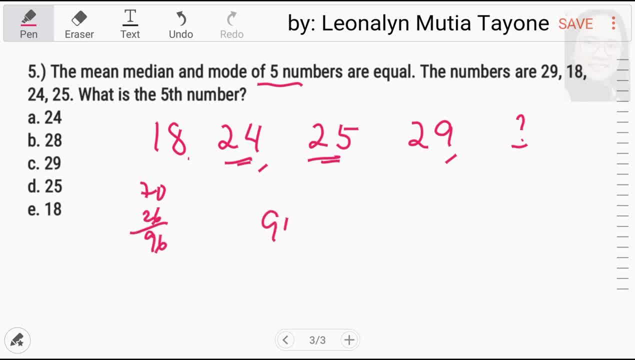 So this is 9 to 6.. Ang total dito ay 9 to 6.. Divided by 4. Kasi apat sila lahat 9 to 6.. 9 divided by 4 equals 2.. 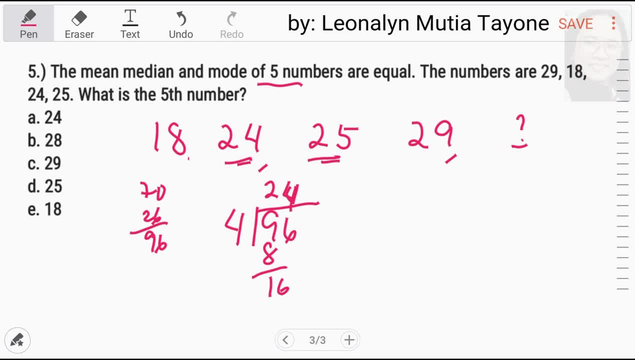 8, tapos 16, 4.. So 96 divided by 4 equals 24.. 24 ang average nitong apat. So ibig sabihin yung panglima ay 24.. I-rearrange ulit natin. 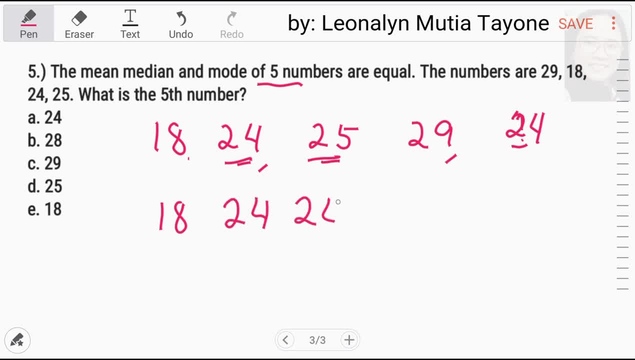 18., 24., 24., 24., 25., 29.. Ibig sabihin, itong lahat naman ito. apat na numbers. Ang average dito ay 24.. Itong lima na na numbers. ang average dito ay 24.. 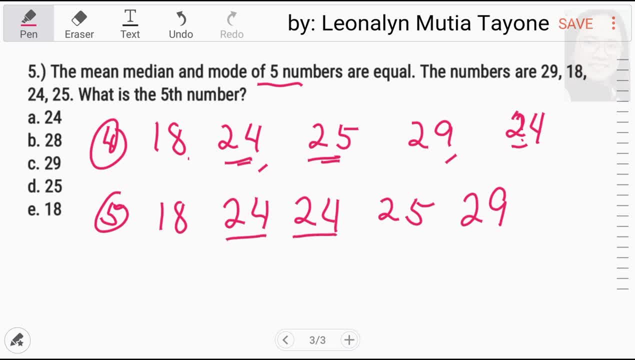 Ngayon. ito yung mode natin 24.. Ang mean natin ay 24.. Ang median natin ay 24.. So ang sagot dito ay letter A. I-emphasize ko lang sa mga nalilito: 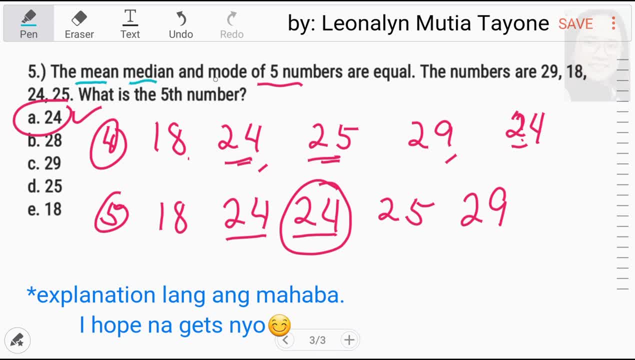 Mean median mode. pareho lang daw itong limang numbers, Kaso ang given apat na numbers lang. Wala namang mode nandyan, So ang mas madali mong gawin ay kunin mo yung average sa apat. 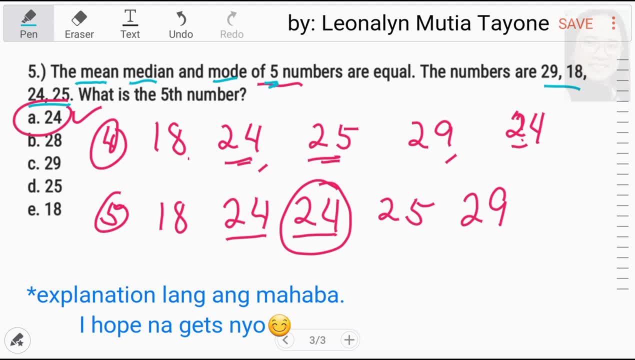 At yung sagot na yun, yun na yung mode. Kasi mauulit dyan, yun yung mode nauulit. So kung nauulit siya, kung ano yung average sa apat? 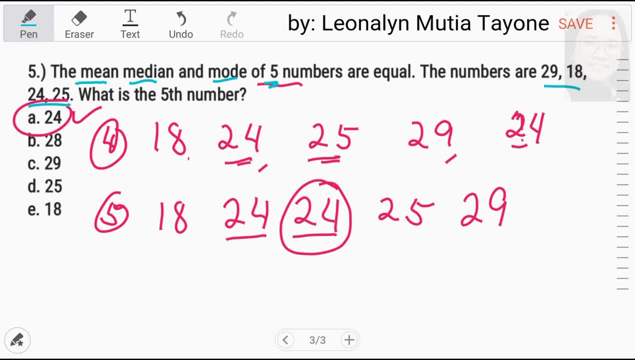 pag lima yung panglima mo, ganun din yung mode, Ganun din yung number na yun. Kung average dito sa apat ay 24, yung 24 na yun, yun yung idagdag mo dito.